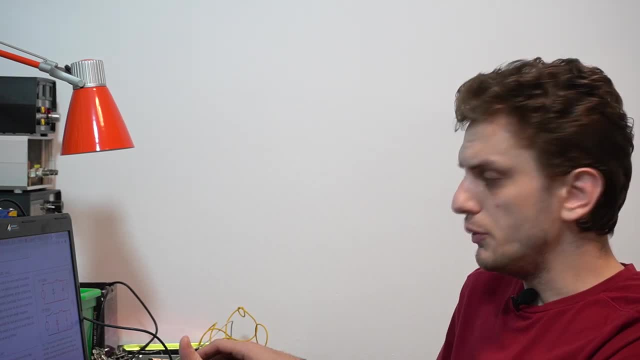 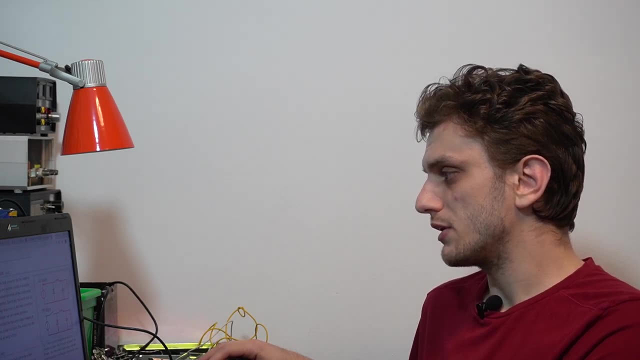 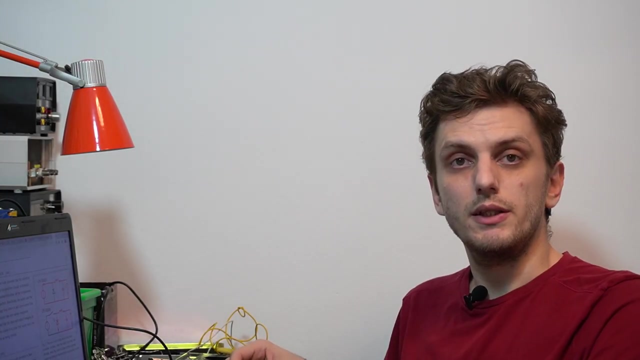 so what we got here on the wikipedia page about it. we see that it's quite a simple circuit. So you got your input supply, output load, a diode, an inductor capacitor and a switch. Now the way it's represented here in this schematic is by a mechanical switch, But in real 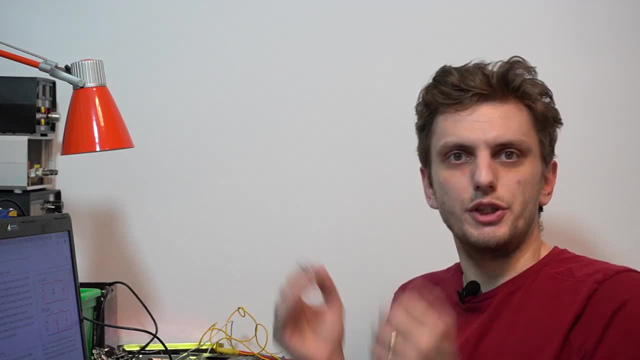 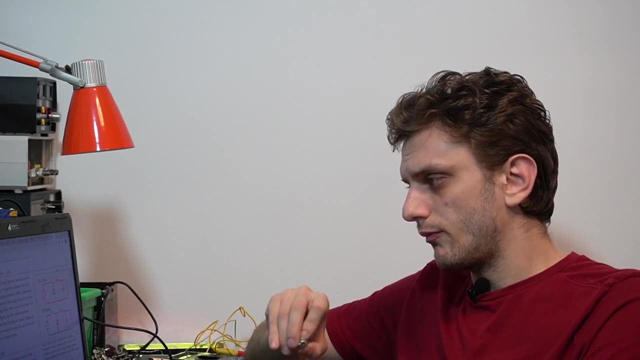 life you're not going to be building your converter with mechanical switches. I mean, you could try, but that's not going to work out very well and you're probably a normal person, so you're not going to go into that. On the other hand, what you will do is replace this switch with a mechanical. 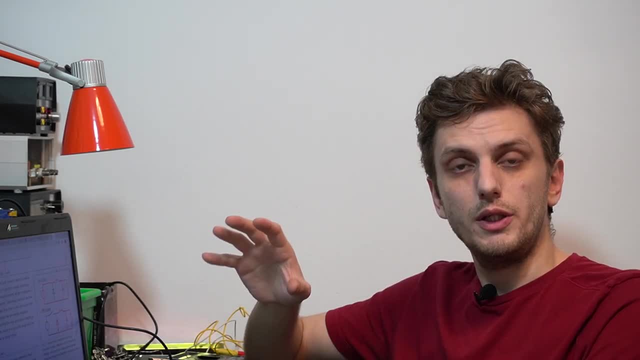 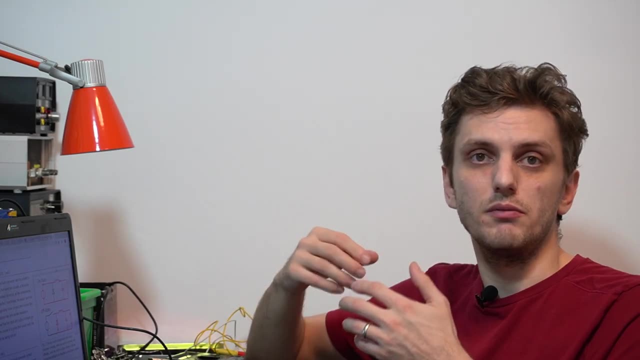 switch with an electronic switch, And what I want to do today is look at the ways you can actually drive the high side transistor switch. So go over the ways of doing it- the right way and the not so right way. So if you're curious about that, and much more, then keep watching. 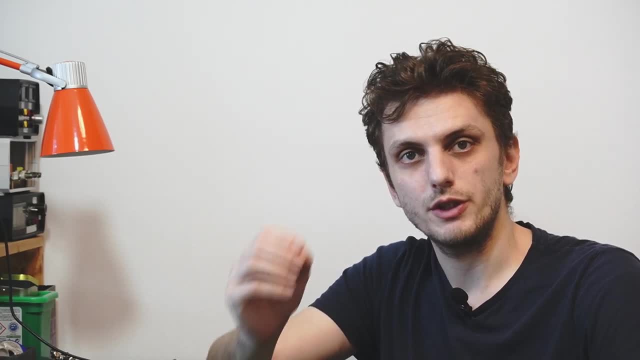 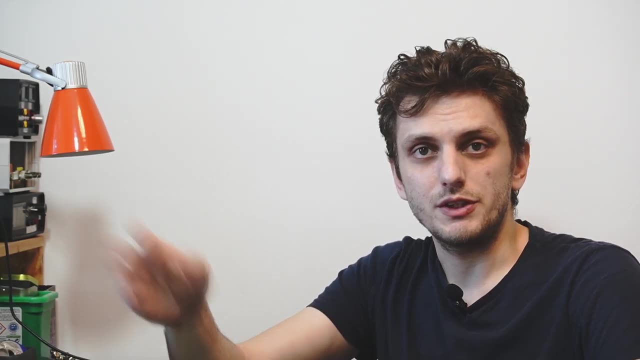 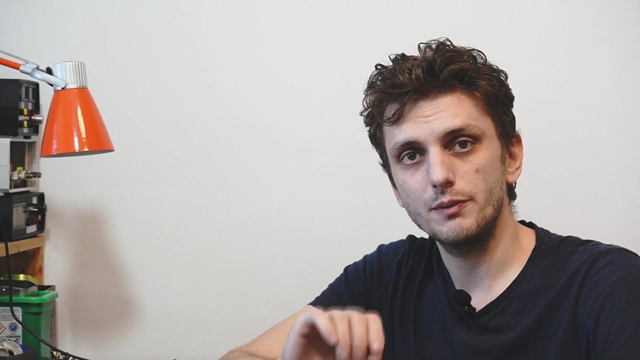 So let's start off by talking about the particular type of transistor used in the converter. Now you can use bipolar transistors, field effect transistors, IGBTs, you name it. you can use any of them in a buck converter, But in particular today I want to focus on MOSFET type of transistors. 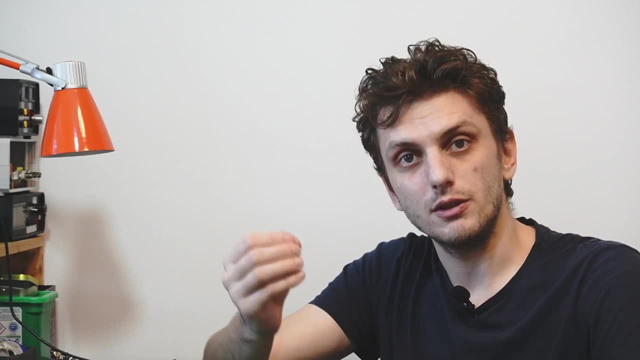 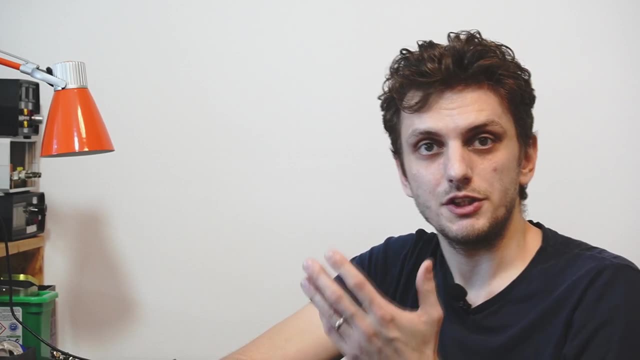 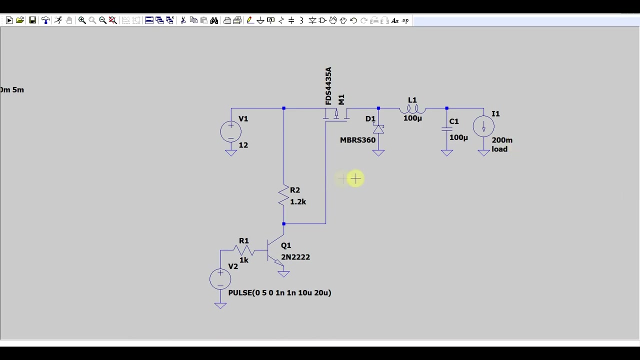 And to start things off, I want to look at how you can use a p-channel MOSFET as a high side driver in your buck converter, And for that let's turn to the circuit simulator LTSpice, of course. So what I got here is the generic power stage for a buck converter using a p-channel MOSFET, of course. 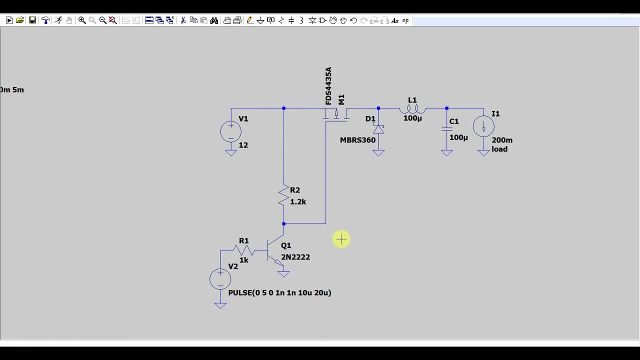 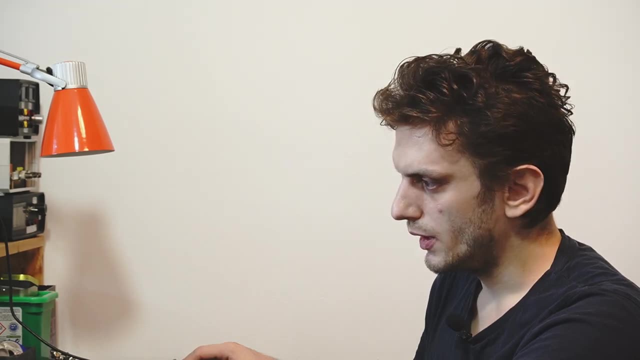 And to drive it I'm using one of the simplest types of circuit you can use. Basically, I'm taking the signal from my signal source and driving it through an open collector type of driver And this will drive the gate of the transistor. And if we run this thing and look at 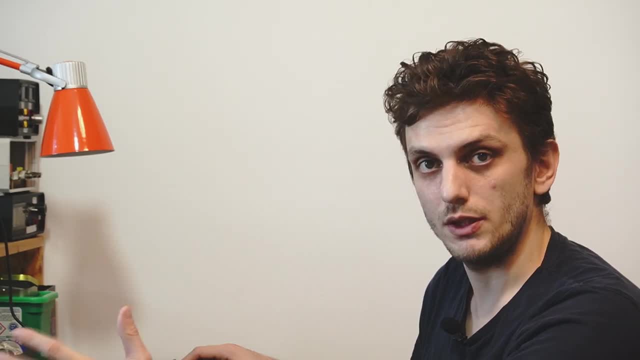 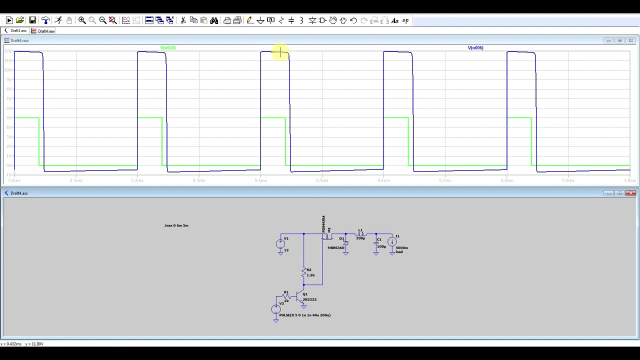 the voltage in the switching node compared to the voltage in the transistor, voltage in the input signal. we can see that when the input signal is high, so is the voltage in the switching node, so the switch turned on, and then, when the signal is low, the voltage in the switching 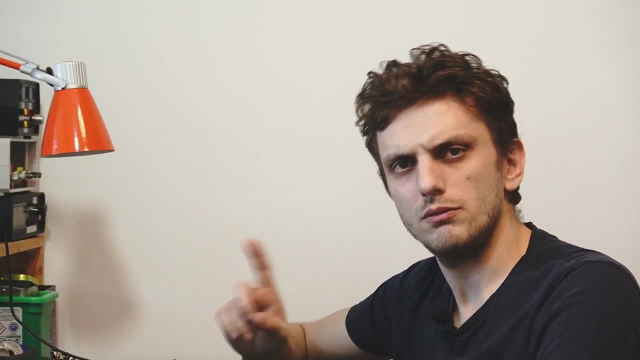 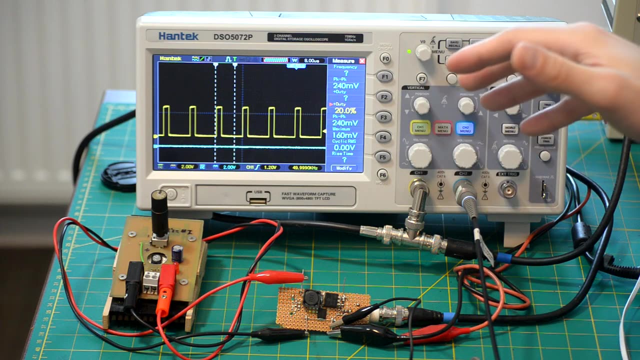 node is low, so the circuit seems to be working. let's just make sure that everything is okay by looking at this circuit in real life. so what i got here is basically the circuit that we've just simulated. i'm taking a signal from the signal generator, passing it through the first channel. 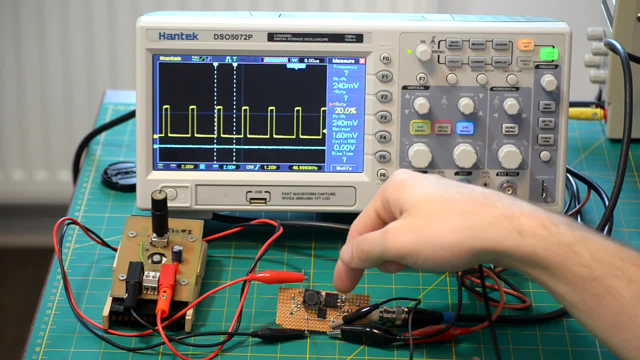 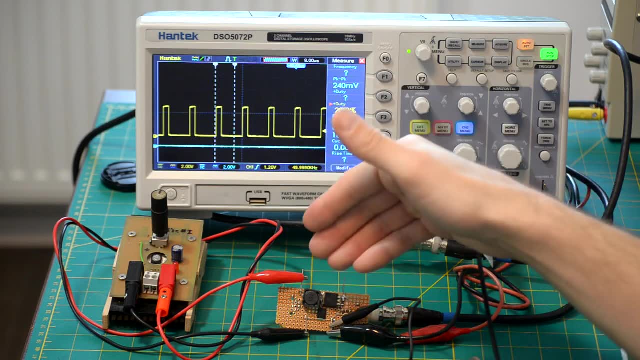 just so we can see it on the oscilloscope, and then using it to drive my high side b channel transistor, then i have the entire power stage of the block converter and then this is connected to an active load on the other side. of course i have some filtering capacitors, but i put them there. 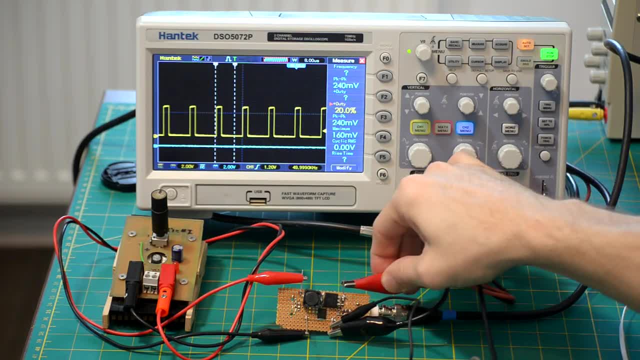 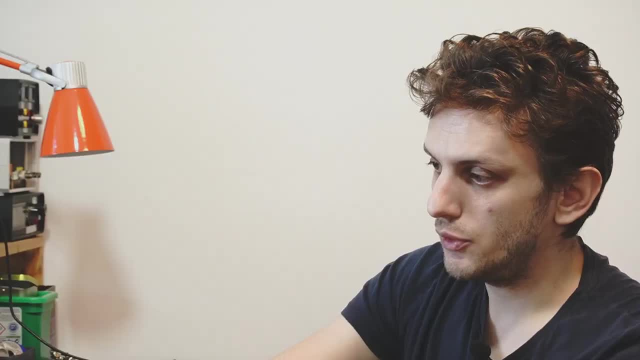 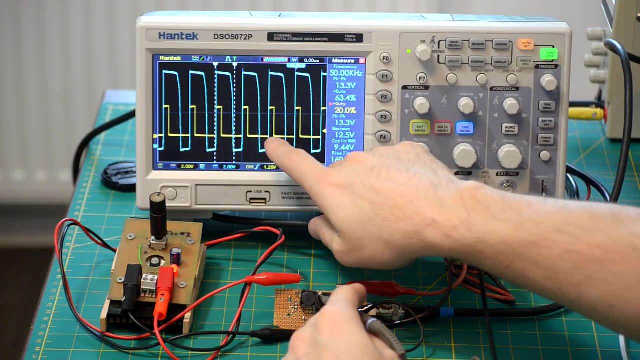 just so that it's nice and tidy. so if we run this thing we see that the active load is on, so seems to be working. and now we can take the oscilloscope probe and look at what the switching node looks like in real life. so we can see, just like in our simulation, that when the input signal is high, so is the voltage in the 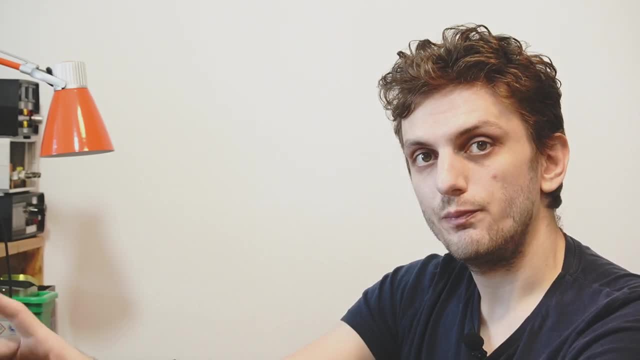 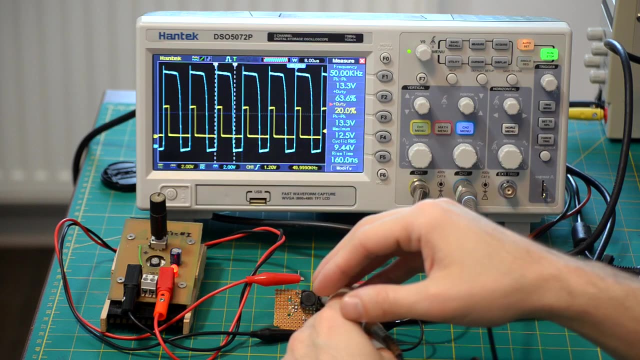 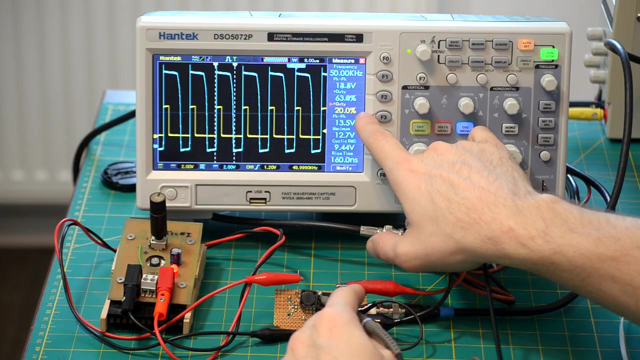 switching node and then they both turn low. but we see one more thing which we shouldn't be seeing: there's quite a lot of delay in between the two signals and this ends up affecting the duty cycle. even though i'm driving the circuit with a 20% duty cycle, i end up having 63% because of this. 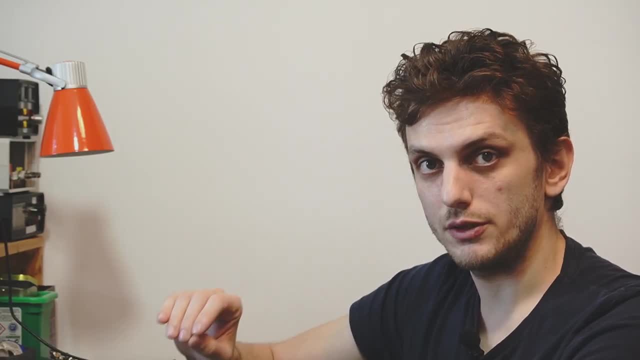 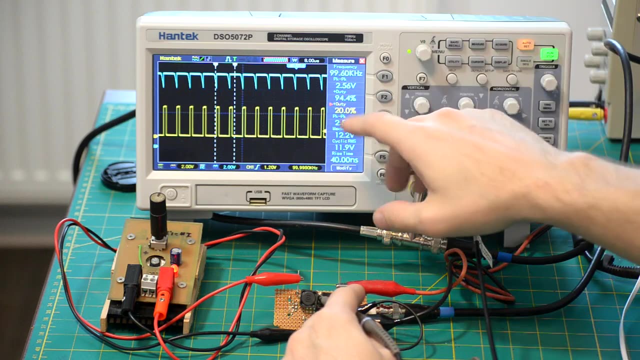 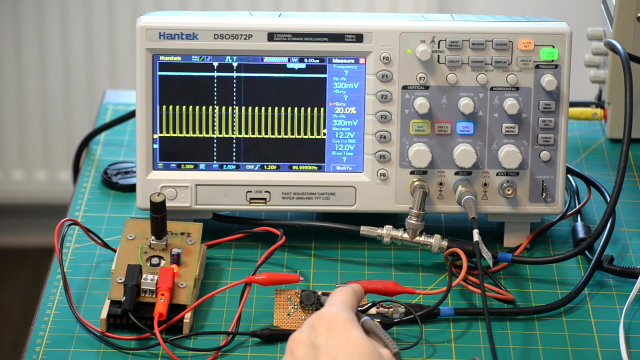 delay. and even worse if i mess around with the switching frequency. say i go from 50 kilohertz to 100, the switch is now barely switching, so you can see that it's trying to turn off, but it's not really getting there. and if i turn up the frequency a bit more, go to 200 kilohertz. 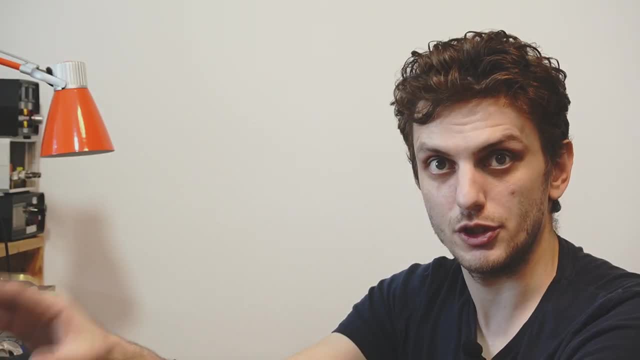 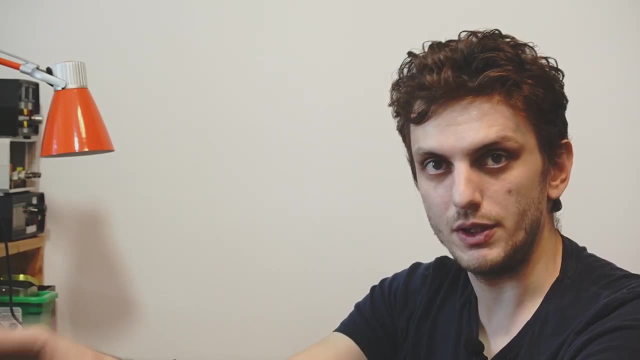 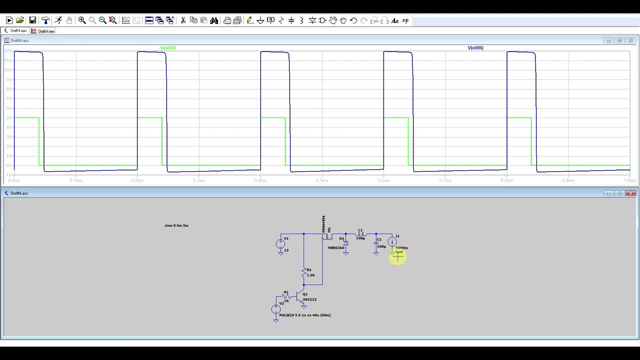 the switch is not completely on, it never has time to turn off, and this is not a good thing. the voltage in the switching node should follow as close as possible the input signal. so how do we fix this? let's turn back to the simulation for this. so the problem we're getting here is that, even though the voltage in the switching node turns high, almost exactly as the input signal does, 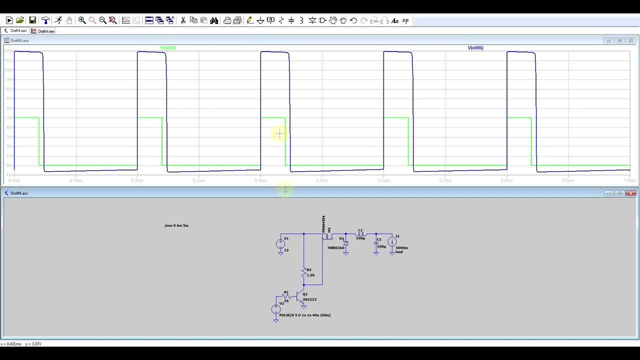 we can't say the same thing about the signals going low, difference being that to pull the signal high, you need to turn on the transistor, and you're doing this using the low side transistor in the circuit, whereas to turn it off relying on this resistor. So the easiest way to fix this problem is to go from an 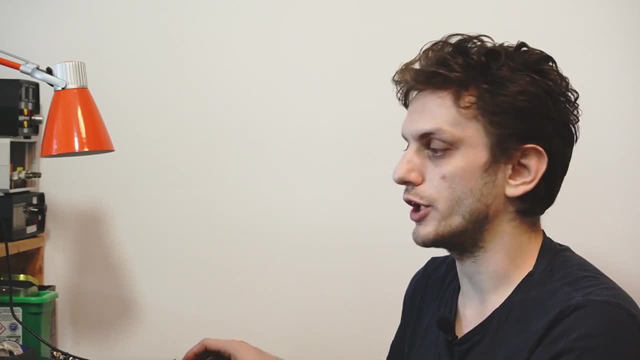 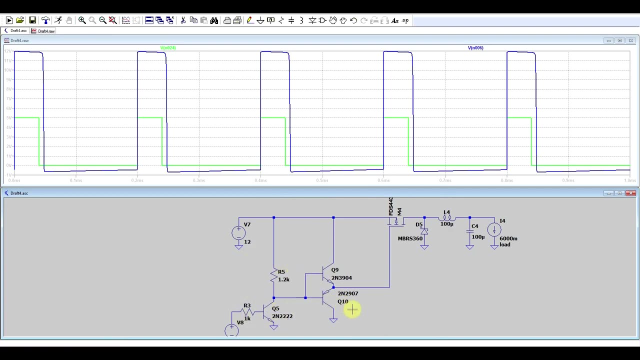 open collector type of driver to a push-pull type of driver, Basically what I've got here. So I kept the open collector type of driver, but I'm using it to drive a class B amplifier which works like a push-pull stage By doing: 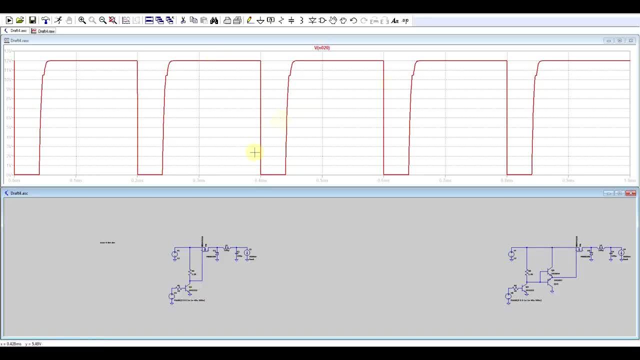 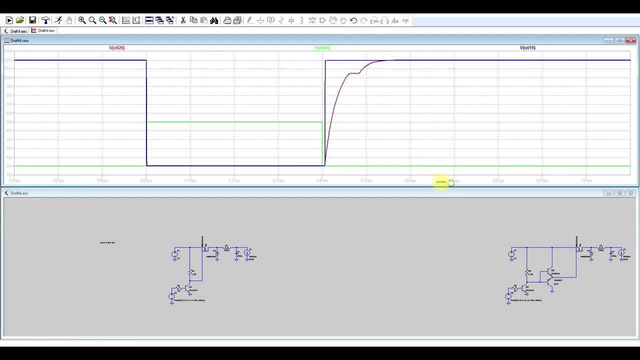 this: the voltage in the gate of the transistor turns from this sort of shape that we had in the first case to a completely different shape. So now we can see that both the turning on and the turning off parts are very clear and very sharp. You don't have this slow turn off phenomenon, and that is because we're 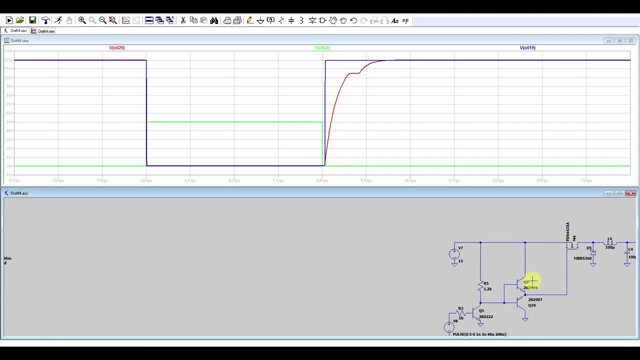 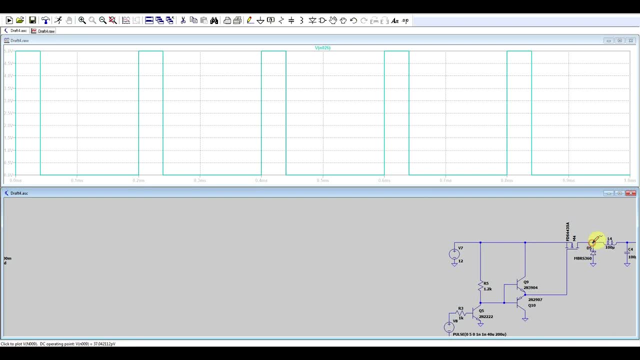 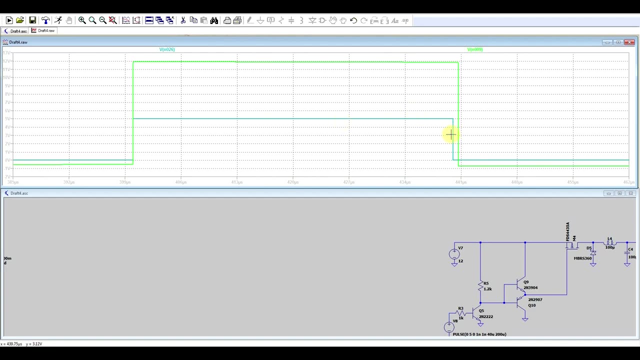 actively turning off the transistor by using the high side transistor, And by doing this we can now compare the input signal to the signal in the switching node And see that we have a very nice, very straight edge. So we still have a bit of delay. That's because the components have a bit of turn on and turn off delay and 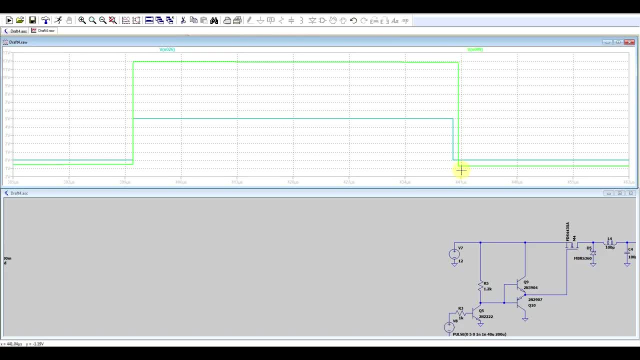 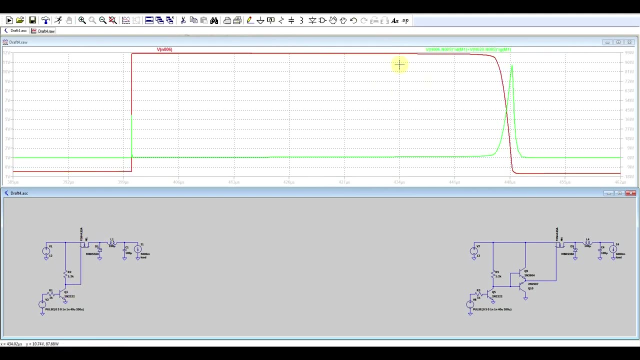 that's perfectly normal, But at least the edges are nice and sharp. And the most important benefit of doing this is that it improves power dissipation. So if we look at our first circuit during this turn off phase, so when the voltage in the switching node goes low, the power dissipation is quite high and 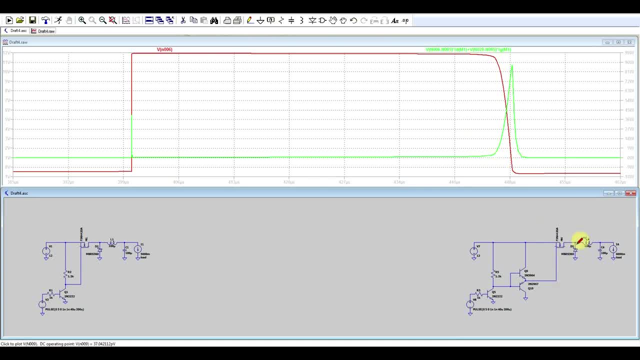 for quite a lot of time. On the other hand, in the second case, if we look at the moment in which it turns off and we look at the power dissipation, we can barely see a very thin line in here. So if we zoom out and compare the power, 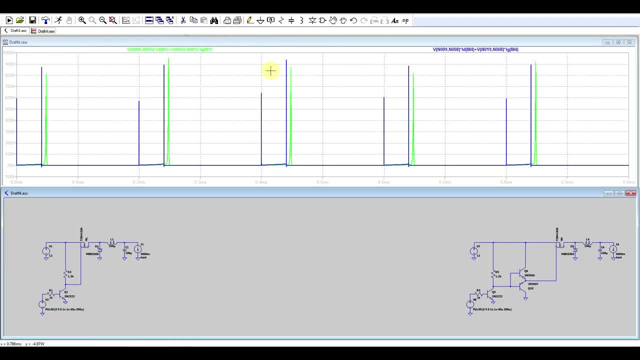 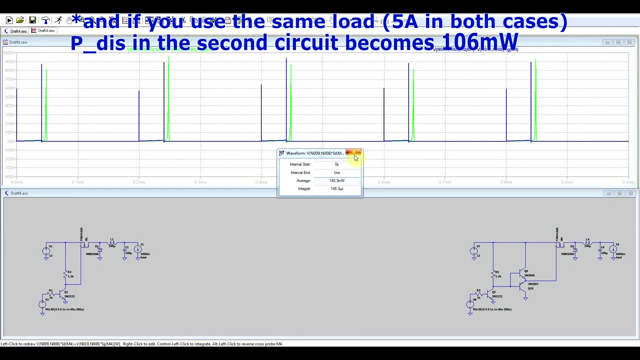 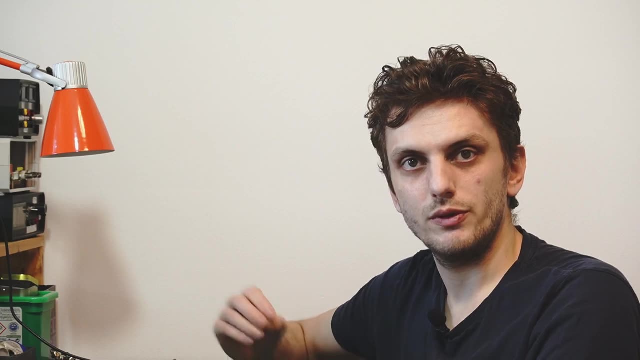 dissipation on the two transistors, the first case and the second case. in the first case we're dissipating around 600 miliWatts, whereas in the second case it drops down to 148. So by improving the switching of the transistor you can greatly improve the converter's efficiency and 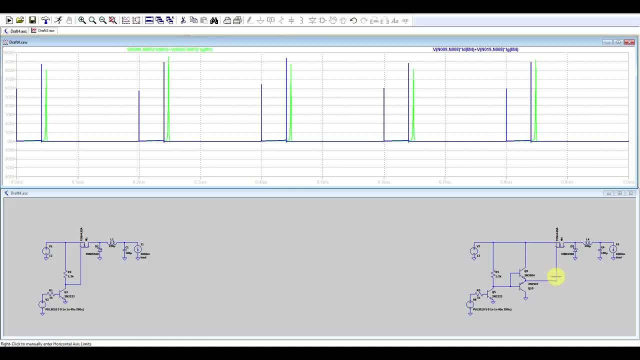 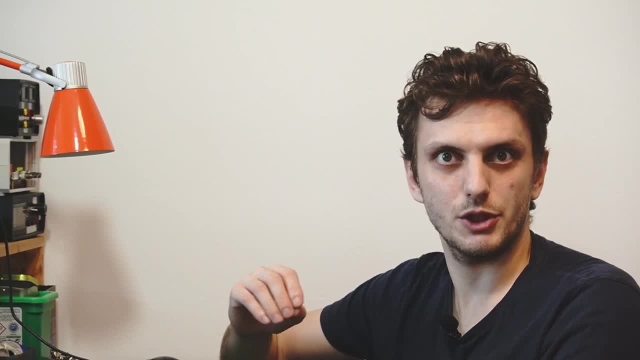 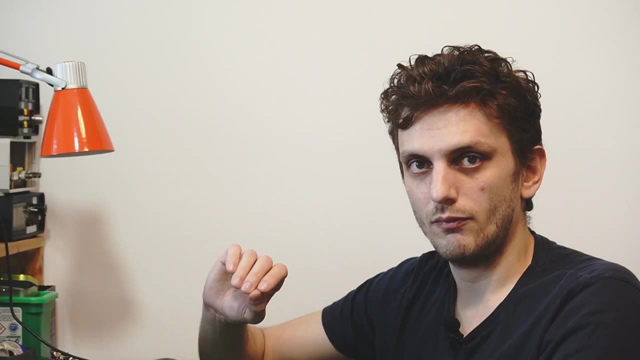 this is basically how you should drive the high side P channel. So using this sort of push-pull driver, you can drive the transistor at much higher frequencies and much more efficiently. The open collector type of driver can work if the switching frequency is extremely low. Now, this about covers the main ways to drive. 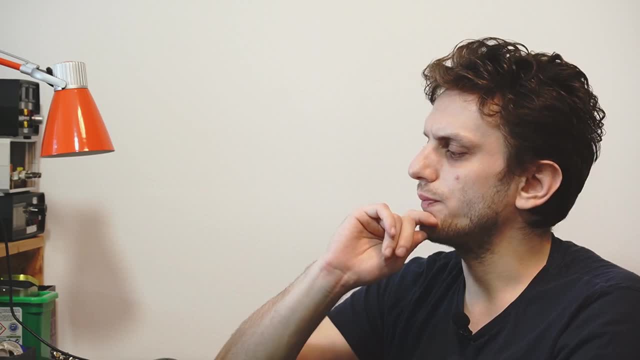 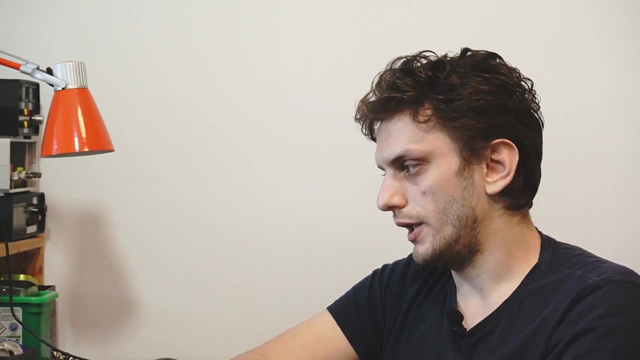 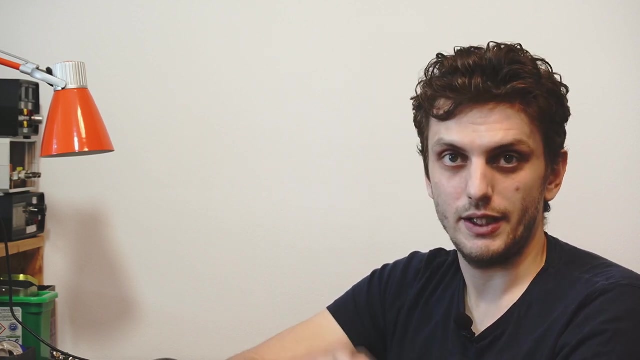 the P channel. but what about the N channel transistor I mean? normally in converters you will find N channel type of MOSFETs, not P channel, and the reason for that being cost related. It's much more expensive to make a P channel transistor than it is to make an N channel transistor, and that is because 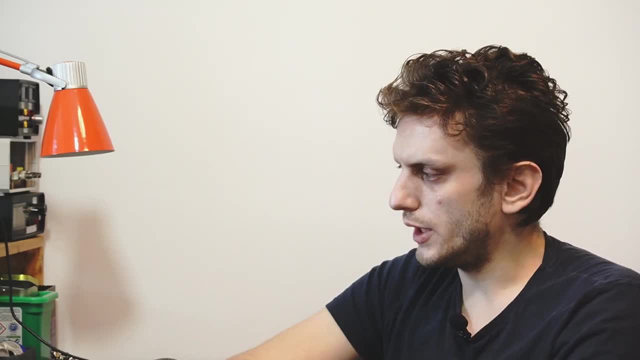 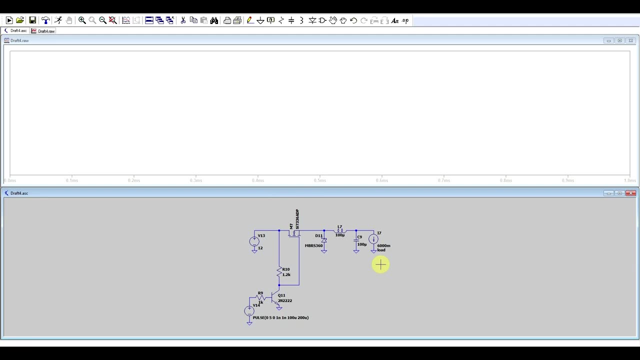 of the process of making it. So let's look at how you can drive N channel transistors now, And here we can see the basic circuit: a built with an n-channel transistor. it looks quite similar with the previous one, the only difference being that i swapped the source and the drain of the transistor, but other than that is the same. 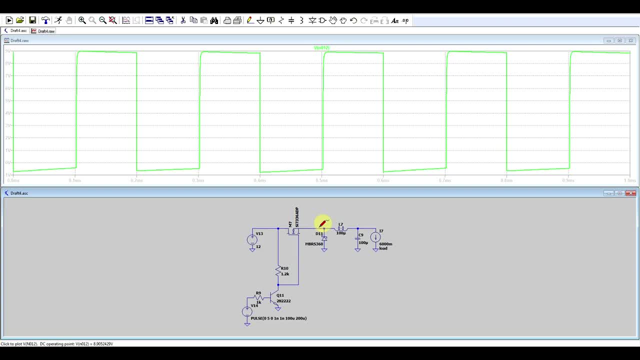 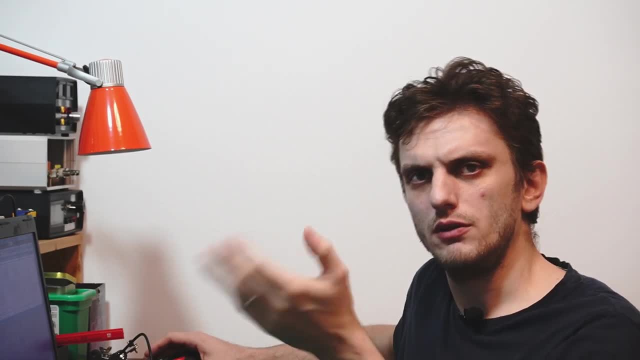 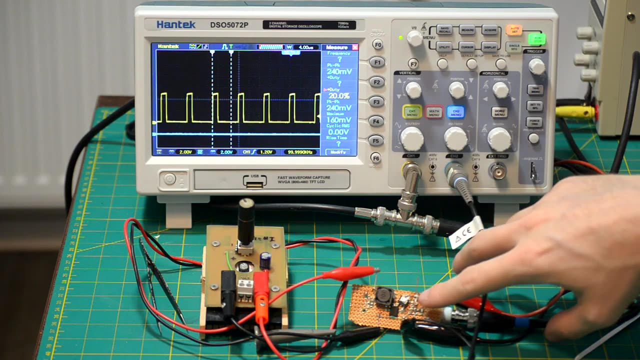 circuit. but does it work well? if we run it, we can see that the switching node is still switching. but let's just see how well this is working in a practical circuit. so what i got here is the same setup as before, only difference being that i swapped the p channel for an n channel. and if 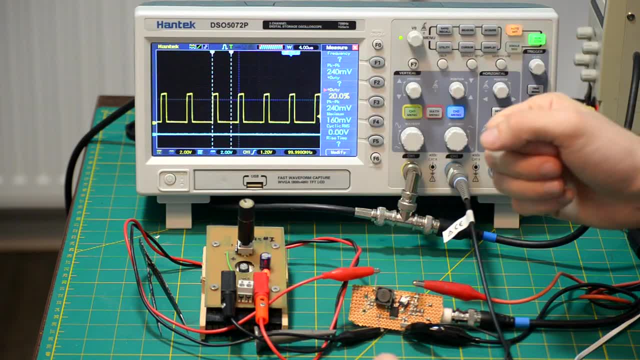 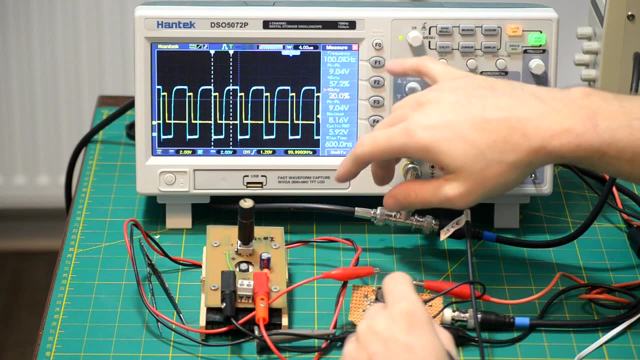 we run this thing, we see that the output is working and if we look into the switching node, just like we've seen in the simulation, it's switching, difference being that this time we have an inverted switching node compared to the input signal. that's because we swapped the p. 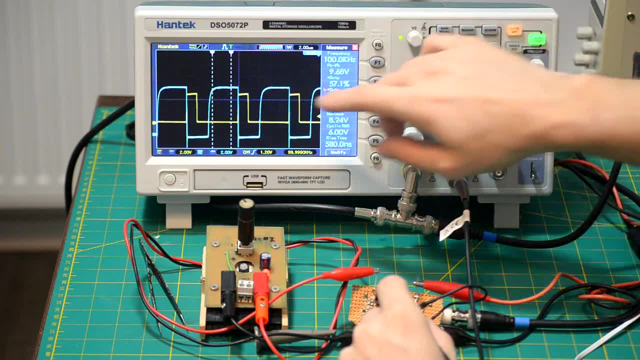 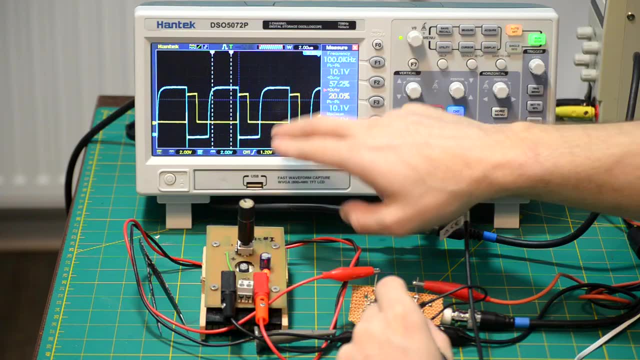 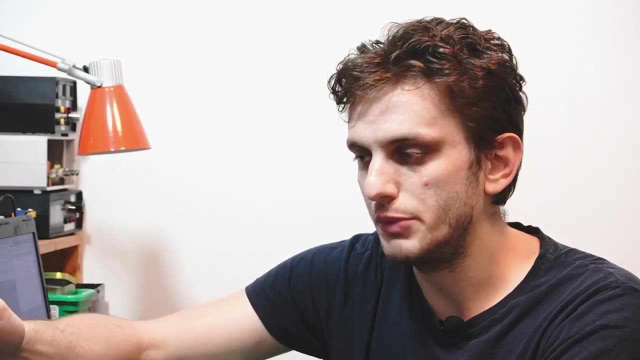 channel. with the n channel we still have this slope going on, so the transistor is not turning on very quick. that can be fixed using the push pull type of driver, and it's important to mention here that the slope at which the transistor turns on when only the resistor is driving it is dependent on. 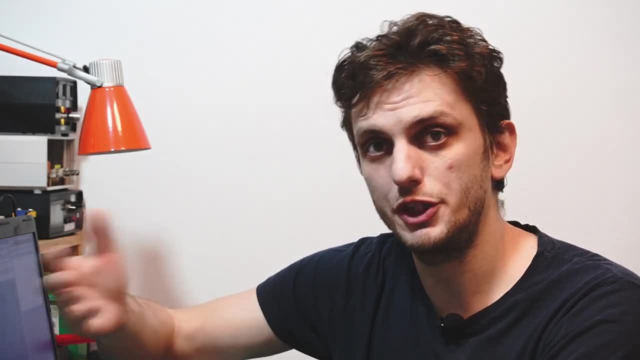 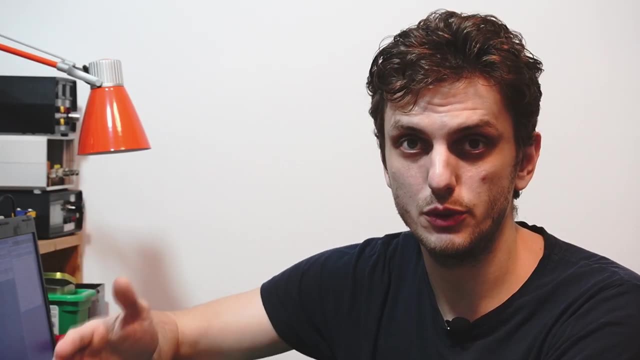 the capacity of the gate. so if you have a transistor with a very large gate capacitance, then it will have a very slow turn on slope. if the gate capacitance is very small, then the slope will be much faster. so there's one more thing you might notice, and that is that the high voltage 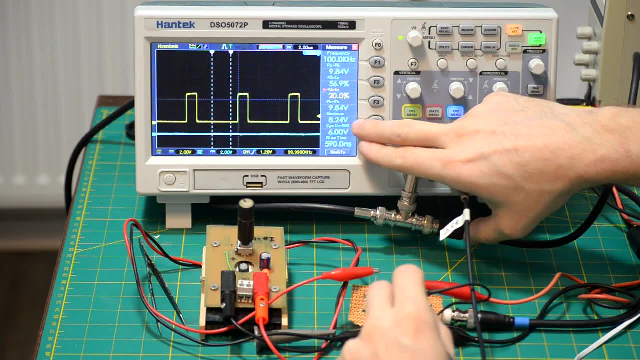 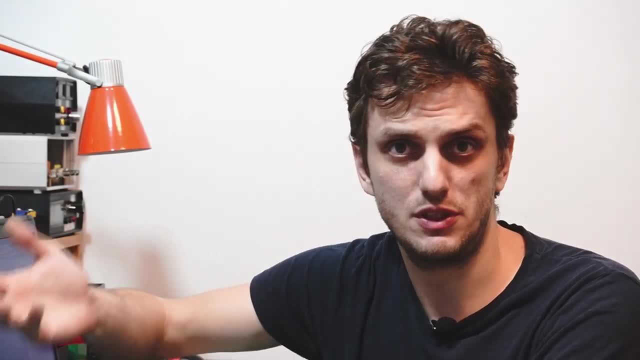 in the switching node is around 8.2 volts, whereas the supply voltage i have it at around 10.. so we've lost 1.8 volts somewhere along the way, and that's not a very good thing. i mean 1.8 volts. 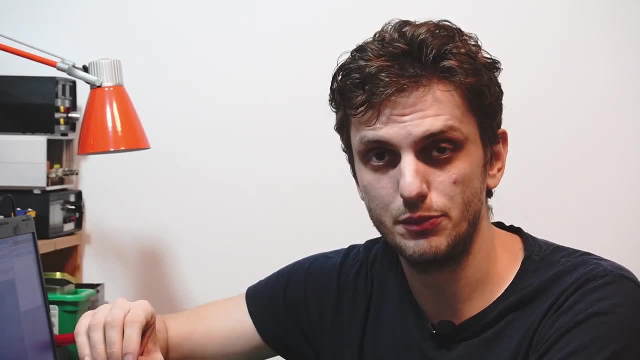 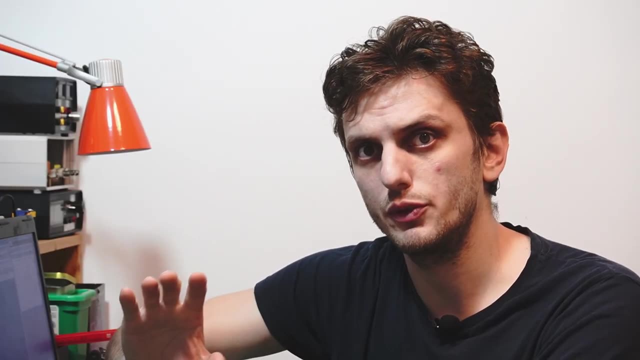 is a large loss and it's completely unacceptable. i mean the slope we can fix with the push-pull driver, but not this. let's go back to the simulator see exactly what's going on. so if we come back here and we look at the input voltage, we see that here we have a very low voltage and we have a very 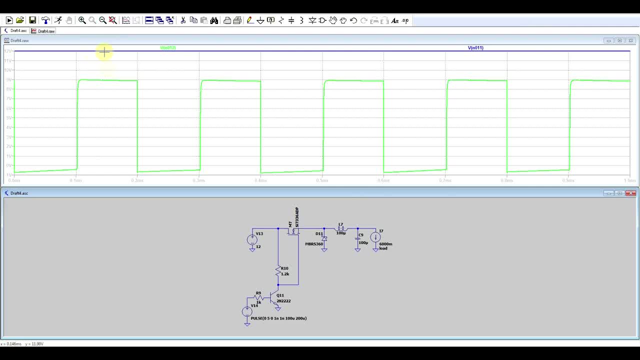 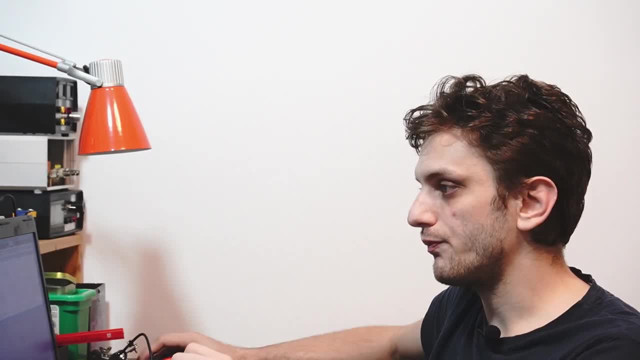 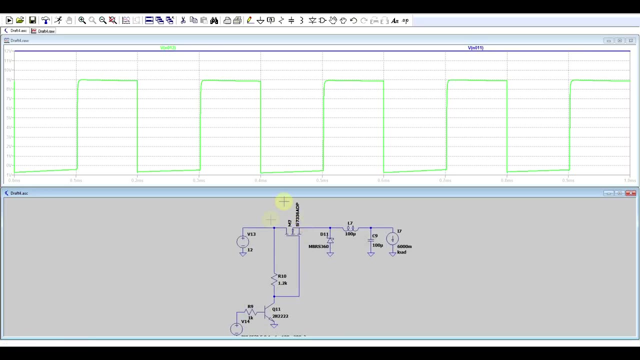 we see that here we have three volts a difference between the input voltage and the voltage in the switching node. now this voltage depends on the exact transistor that you're using and it's the threshold voltage needed to open the transistor. so for the mosfet type of transistor, 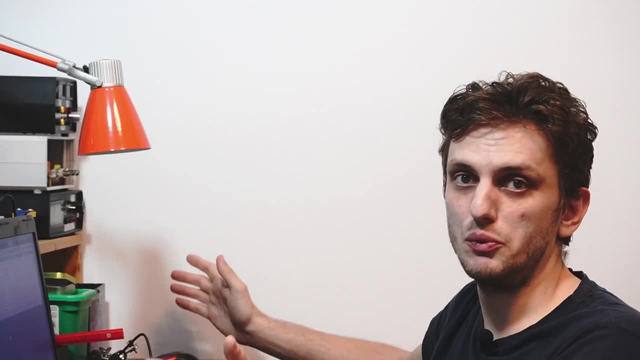 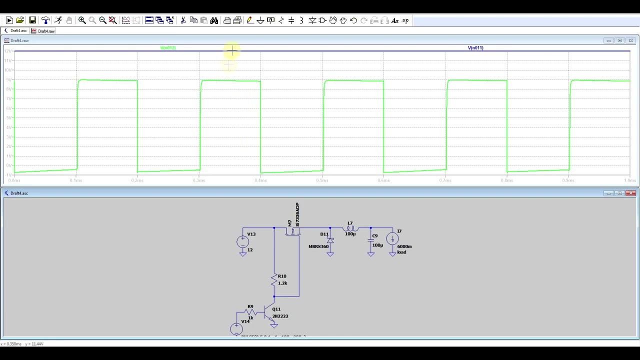 you will have a gate threshold voltage somewhere in between one and three, four volts. highly depends on the transistor. so this particular transistor that i have here in the simulation has a gate voltage of three volts, so the voltage in its source will be 3 volts lower than the voltage. 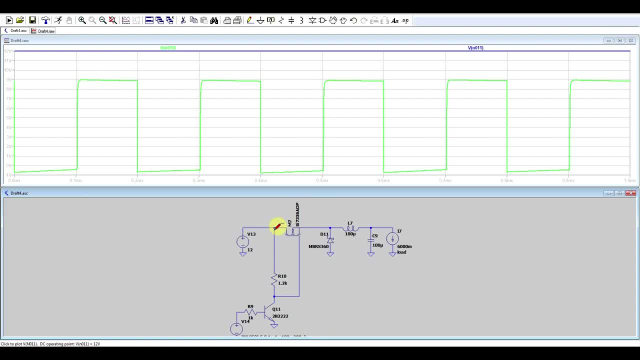 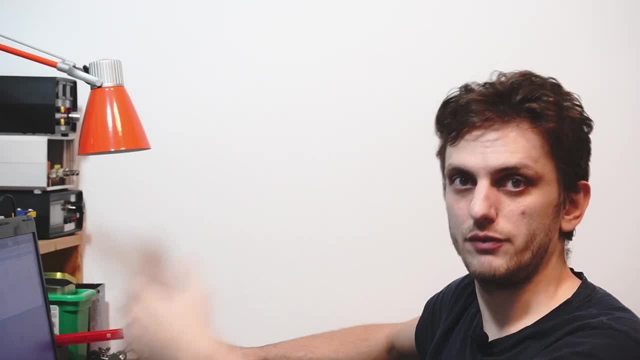 in the gate and the voltage in the gate at the moment has maximum of the supply voltage. so the only way to get this thing, to have a higher voltage in the switching node so to have a very small voltage drop on the transistor, would be to drive the gate with a higher voltage than the 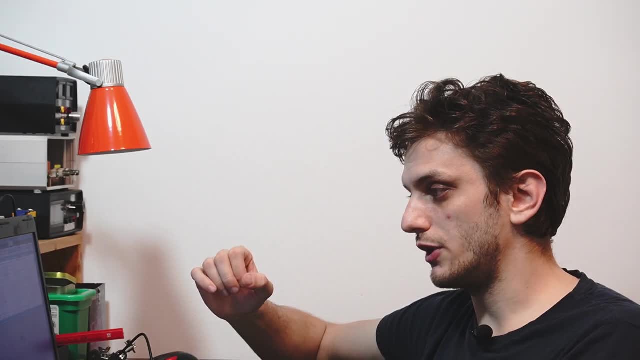 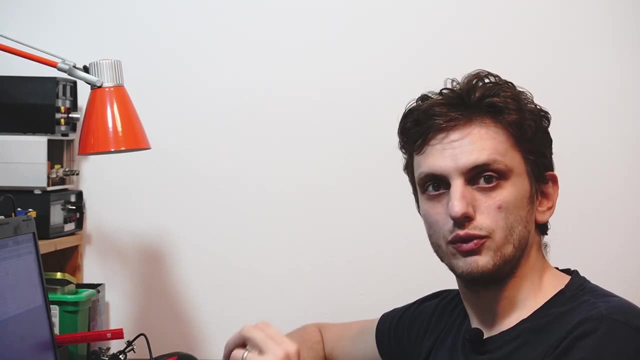 input supply voltage. so if i'm supplying the circuit at 12 volts i will need 15 or 20 volts or something that is more or less 3 volts. so this crush on the transistor will block the structure than 12, more by the gate threshold voltage at least, and we can get a higher. 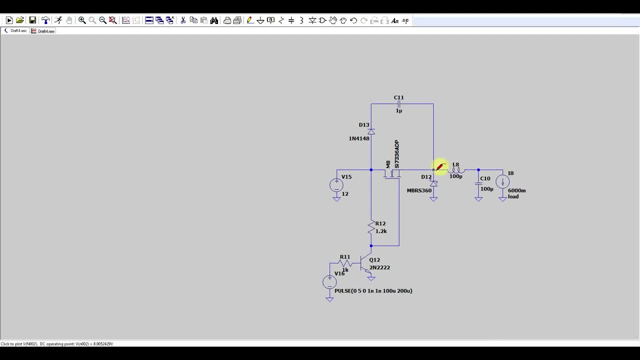 voltage with a circuit like this. So, compared to the previous circuit, I added this capacitor and diode, and the logic behind this is that when the switching node is low, so at 0 volts or lower, then the diode will charge the capacitor. When 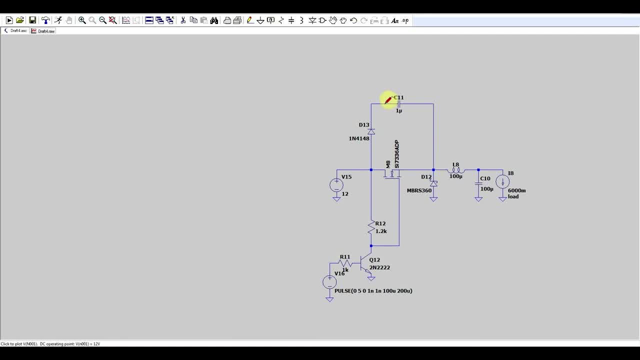 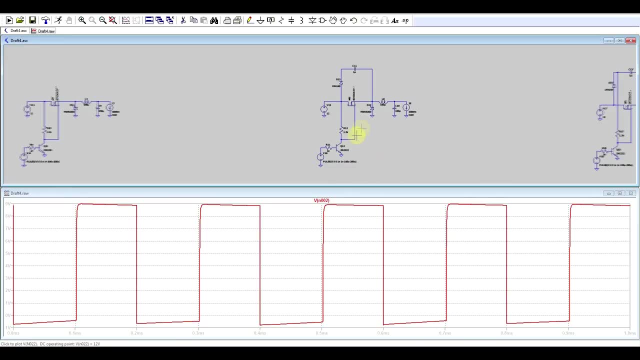 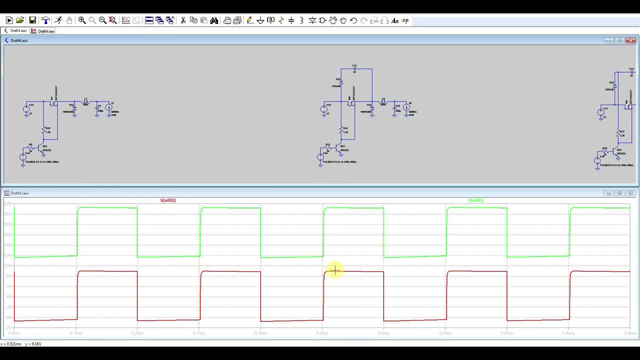 the voltage in the switching node is high, then the voltage on the capacitor would be higher than that of the input voltage. This is also called a bootstrap capacitor, and if we look at how this works so we can see that the voltage in the switching nodes goes up to 9 volts, but the voltage on the capacitor at the 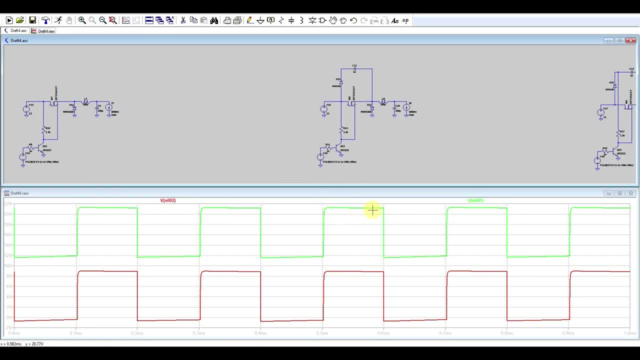 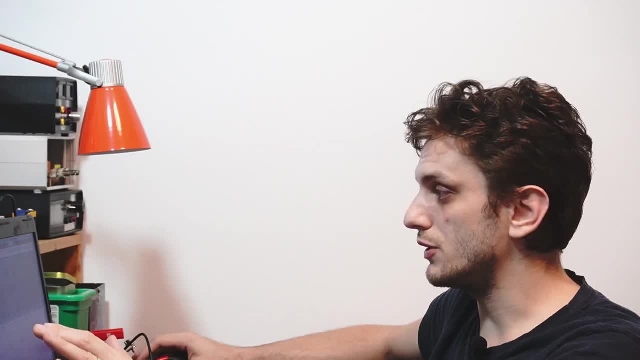 moment when the voltage in the switching node is high gets up to 21 volts, So plenty enough to drive the transistor. So there's just one small modification that needs to be done to the circuit, and that is connect the high side resistor to.